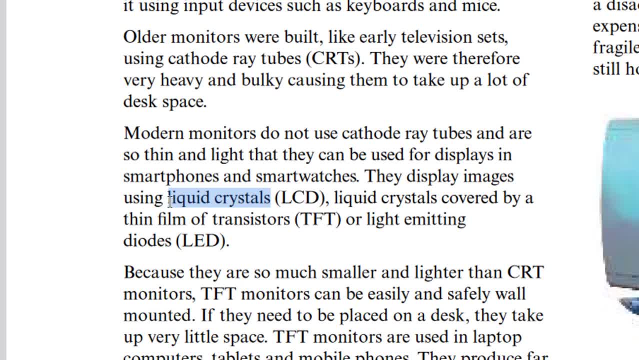 The. they display images using liquid crystals. Liquid crystals, ergo LCD, Liquid crystal display. LCD: Liquid crystals covered by a thin film of transistors. They are called TFT or light emitting diodes, LED. So in LCD either we have TFT or LED light emitting diodes. Okay, so enough about. 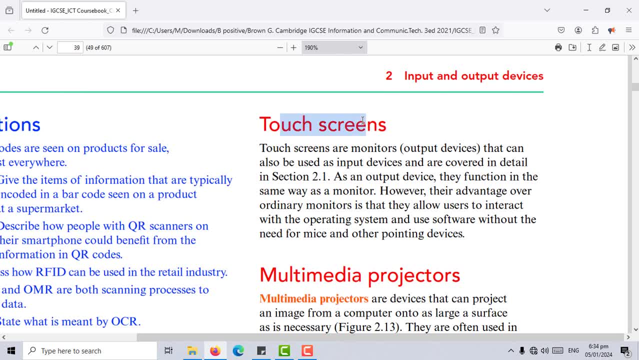 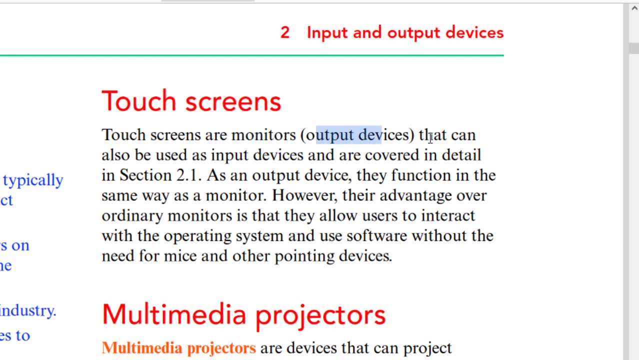 um monitors, let's go to touch screens. since we're talking about monitors, Touch screens are monitors and the monitors are output devices that can also be used as an input device and are covered in details later. They function in the same way as a monitor. however, their advantage over ordinary 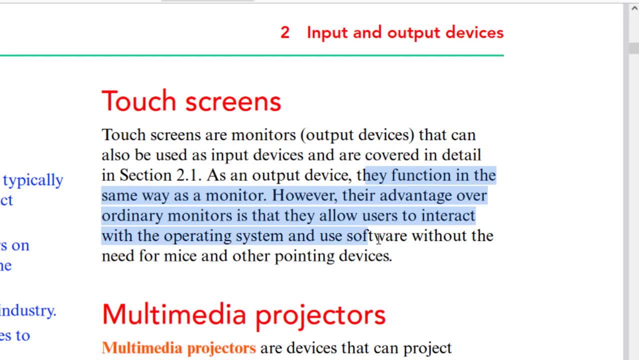 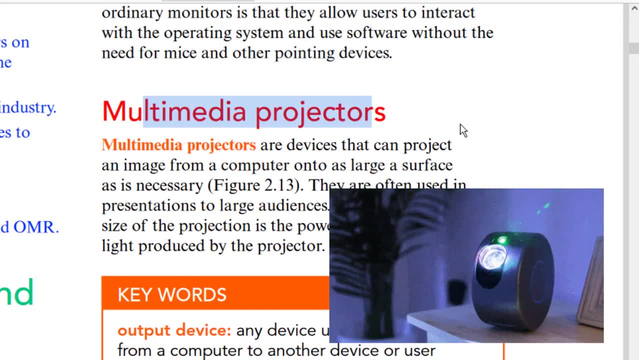 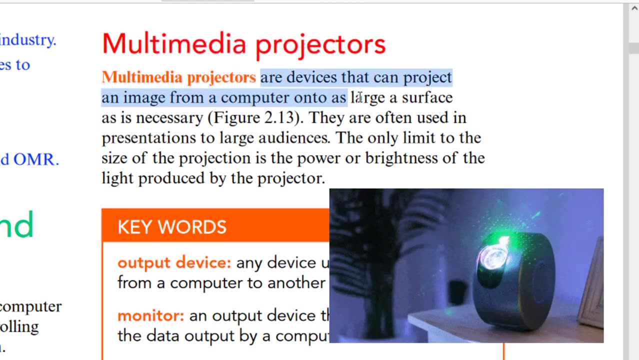 monitors is that they allow users to interact with the operating system or the software without the need for a mouse or a pointing device. Moving on to multimedia projectors, Multimedia projectors are devices that can project an image from a computer onto a large surface or in a large wall or wherever. 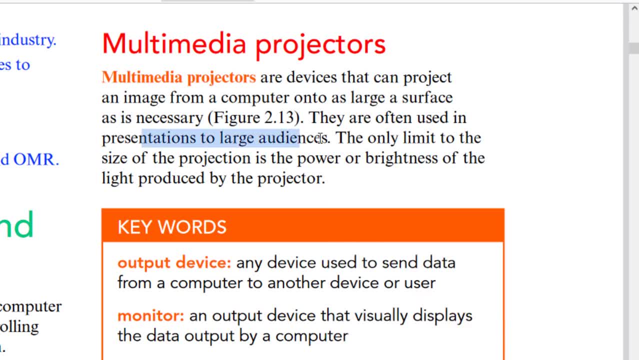 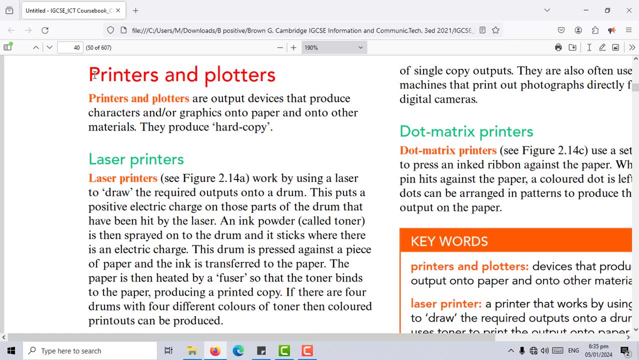 right, they are all often used in presentations to large audiences. All right, let's move on to printers and plotters. I'm not going to tell you that plotters are a really, really, just a really really big printer, because I don't want you to write that on an assessment. all right, so? 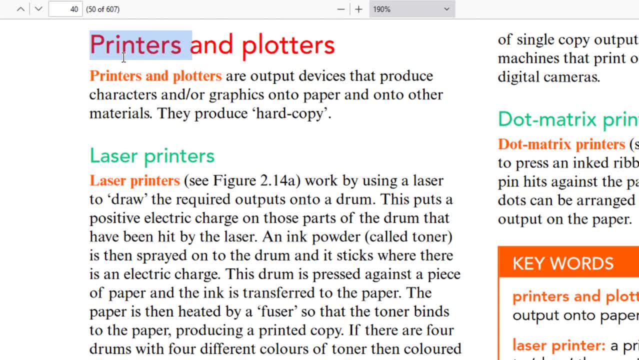 So we mostly are going to use the books word. All right. so printers and plotters are output devices that produce characters or graphics onto paper and onto other materials. They produce hard copy And that is what we're going to put on an assessment, if you were asked about that. 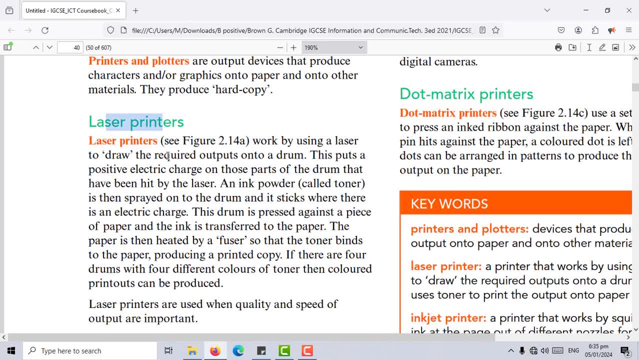 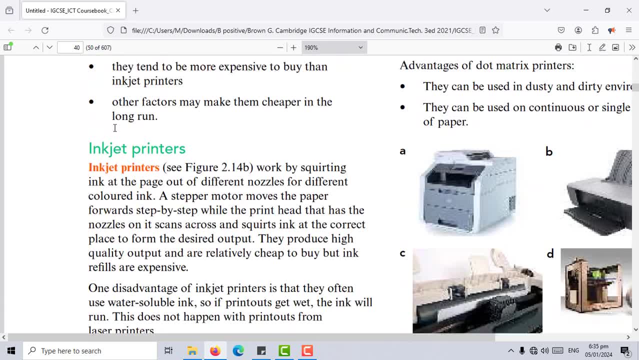 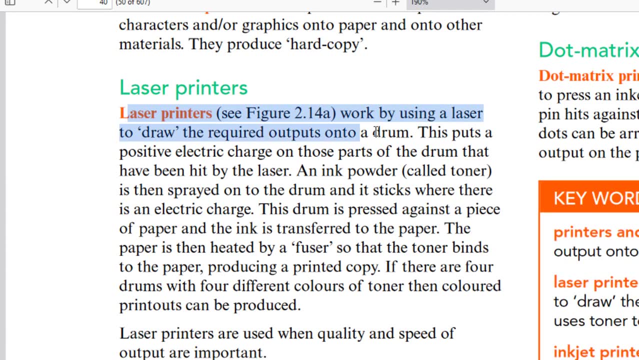 Now we have different types of printers: laser printer, inkjet and dot matrix printers. Laser printer- where is it? Laser printer? Laser printers work by using a laser to draw the required outputs onto a drum. This puts a positive electric charge on those parts of the drum that have been hit by the laser. 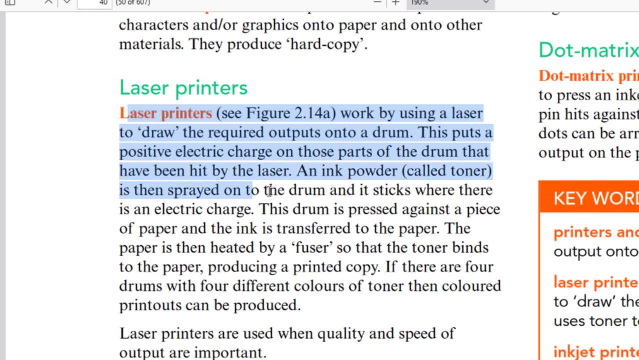 An ink powder called toner is then sprayed onto the drum and it sticks. where there is an electric charge. This drum is pressed against a piece of paper and the ink is transferred to the paper. Basically, that's how laser printer works. They have literally. 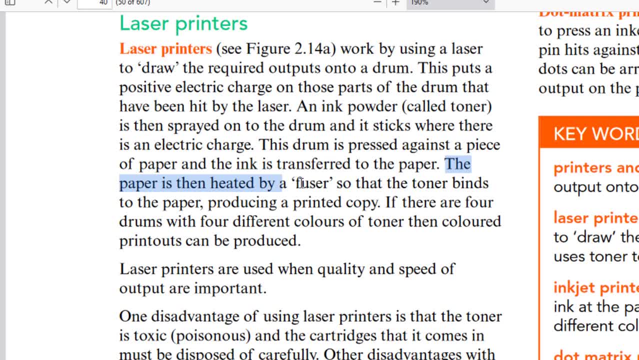 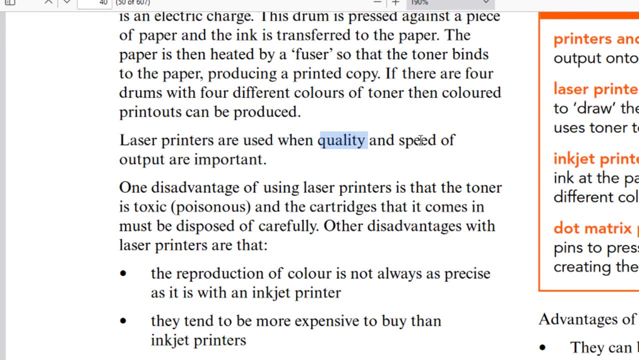 He explained the whole process. The paper is then heated by a fuser so that the toner binds to the paper, producing a printed copy. All right enough with that. One of the advantages of laser printers is that it is used when we are looking for quality and speed. 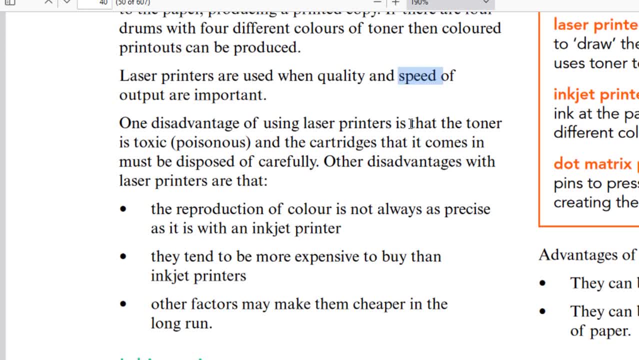 Yeah, Now, one disadvantage of using laser printers is that the toner or the ink is toxic, poisonous, And since it's poisonous, we have to get rid of it very carefully. We need to get when we need to dispose of it. we need to do that carefully. 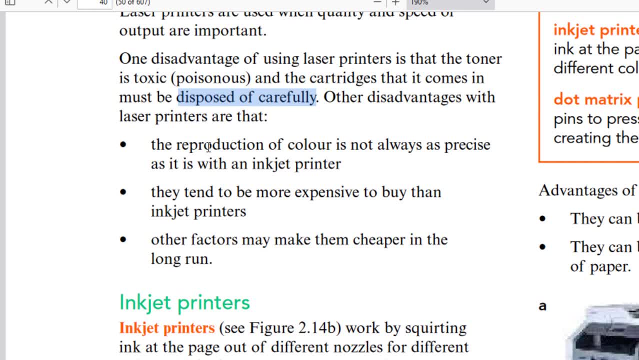 Other disadvantage is that the produced, the reproduction of color is not always as precise as it is with an inkjet printer. So immediately we're going to get from that is that inkjet printers are more clear. They produce more clear hard copy. 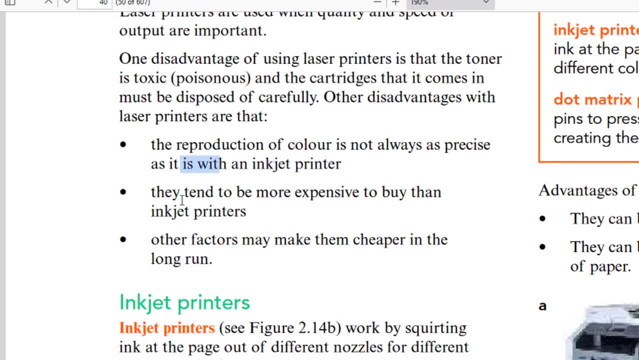 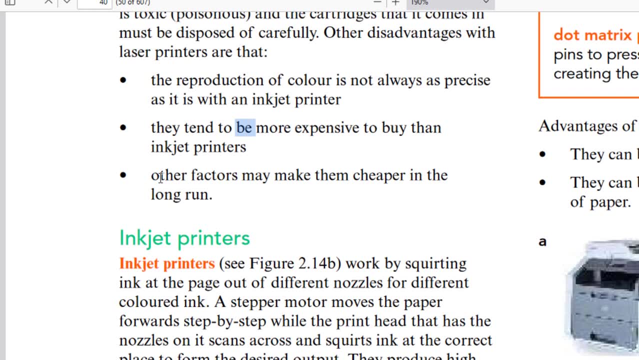 But again, don't Use my words, Use the book's word. All right. They tend to be more expensive to buy than inkjet printers. So money is a factor here. Okay, Other factors may make them cheaper in the long run. 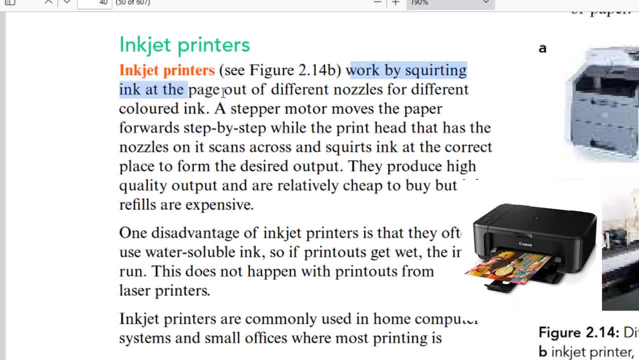 Inkjet printers. they work by squirting ink at the page out of different nozzles for different colored ink. A stepper motor moves the paper forward step by step while the print head, while the print head that has the nozzles on it- scans across the squirted ink, the squirts ink at the correct place to form the desired output. 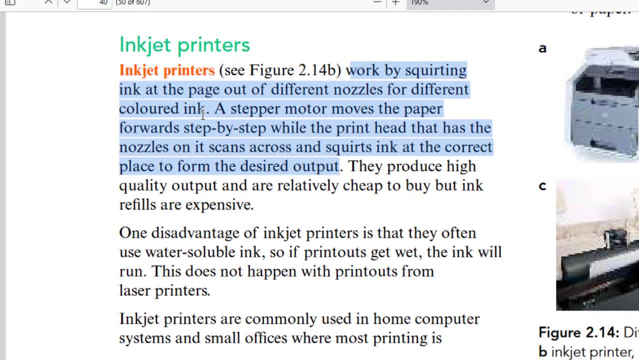 Okay, So another tough definition for another printer type. Okay, So the advantage is that they produce high quality output and are relatively cheap to buy, But ink refills are expensive. That could be a disadvantage. One disadvantage of ink printers is that they often use water. 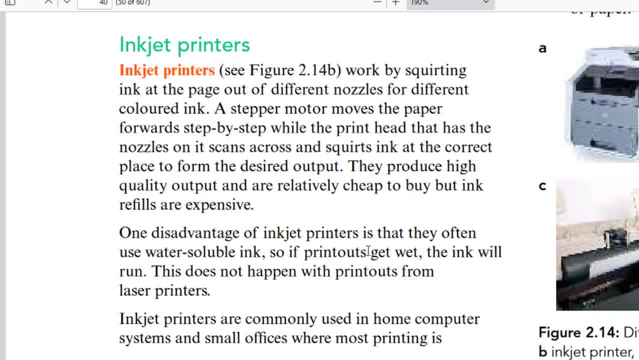 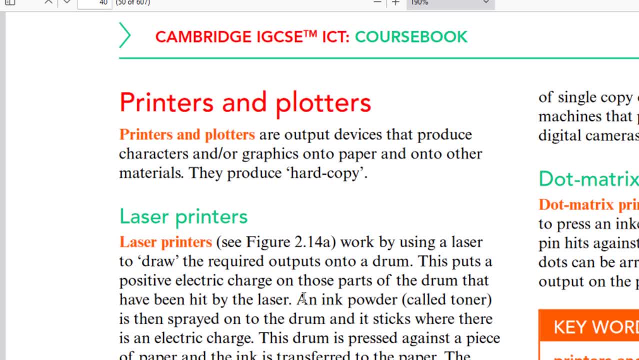 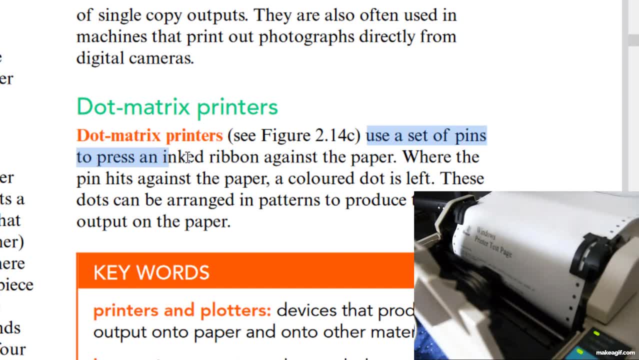 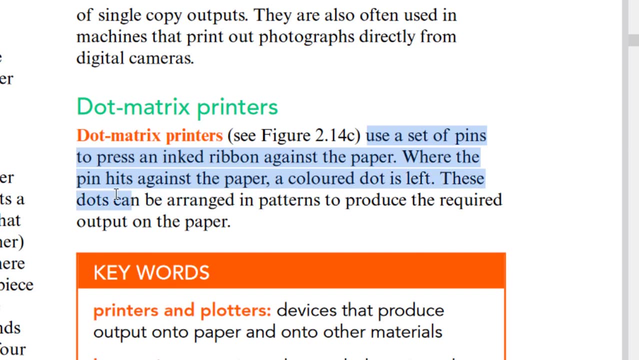 All right, Moving on to the third type of printers: dot matrix. A dot matrix use a set of pins to press an ink ribbon against the paper. Where the pin hits against the paper, a colored dot is left. These dots can be arranged in patterns to produce the required output on the paper. 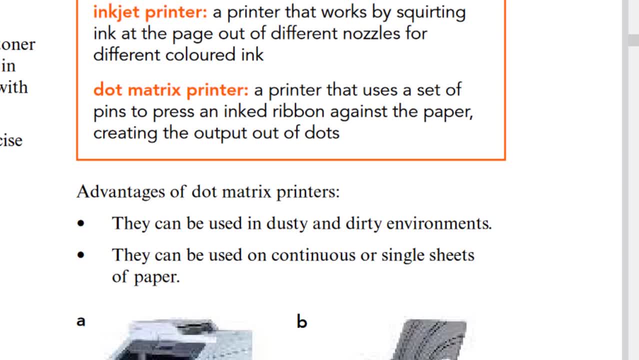 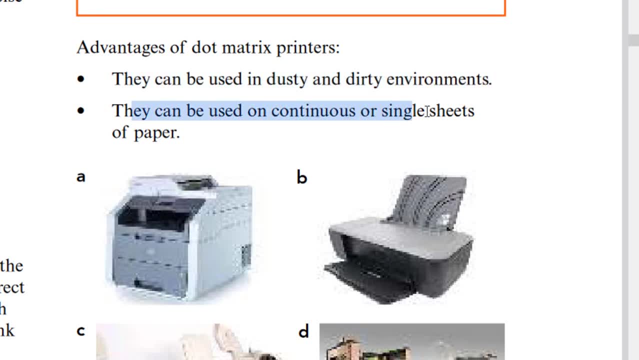 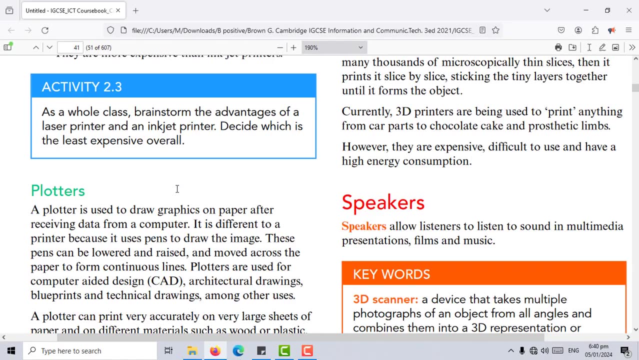 So this is basically the easiest one to understand. right Advantages is that they can be used in dusty and dirty environment. They can be used on continuous or single sheets on single sheets of paper. Now, we're not going to go on and on about the advantages. 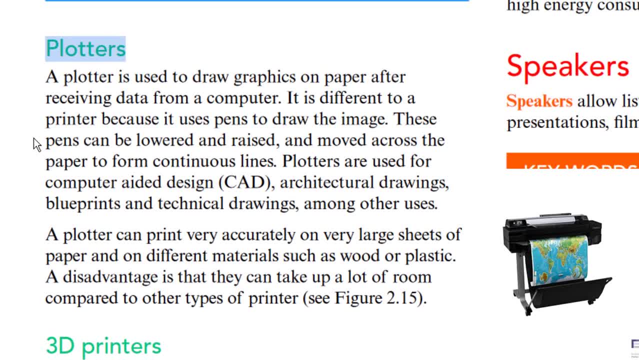 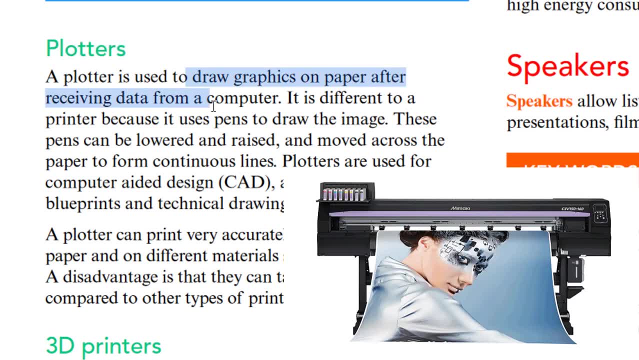 We're going to go to plotters. What are plotters? The question that everybody has Has been asking themselves. A plotter is used to draw graphics on paper after receiving data from a computer, So obviously it's going to receive data from the computer. 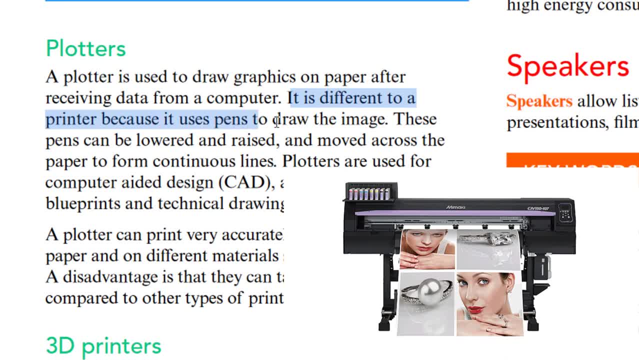 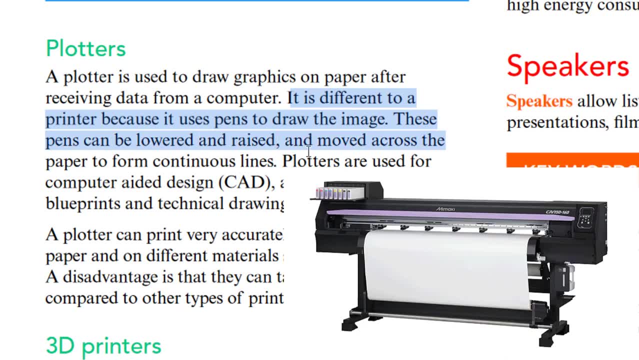 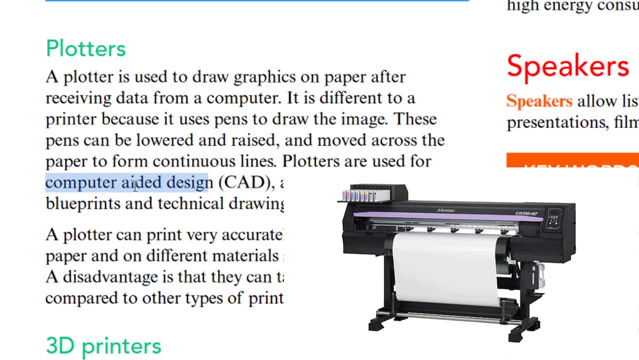 It is different to a printer because it uses pens to draw the images. These pens can be lowered and raised and moved across the paper to form continuous lines. Plotters are used for computer aided designs. If you can remember CAD, It's one of the. 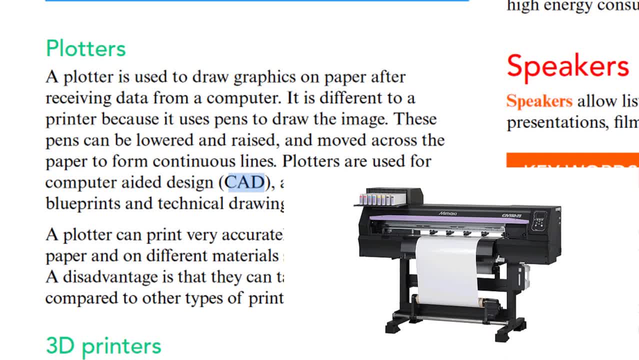 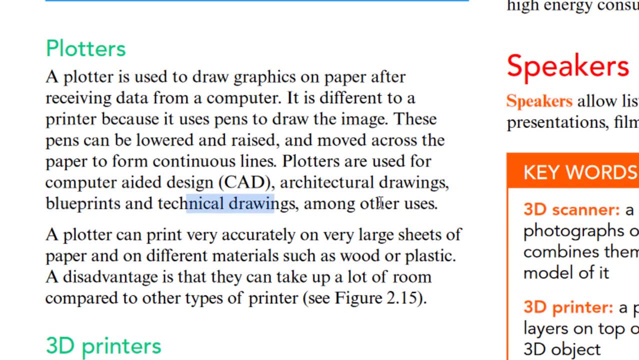 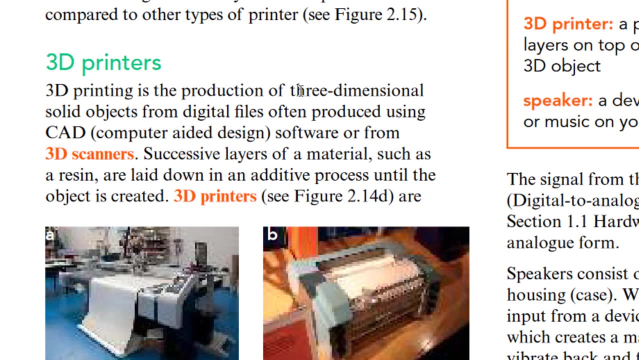 The computer applications that we studied, or the software applications- Okay, so it's used for that- and architectural drawings, blueprints and technical drawings, among other uses. All right, Now let's move to 3D printers. 3D printing is the production of three-dimensional solid objects from digital files, often produced using CAD. 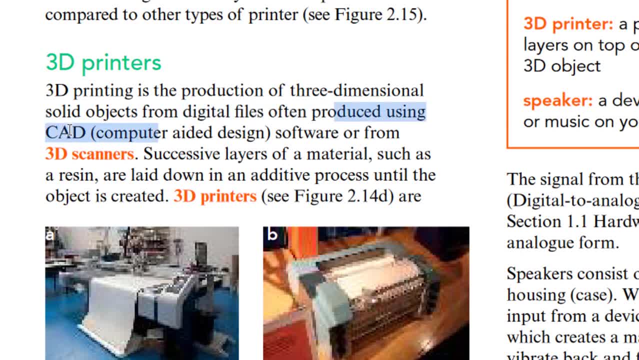 So if we are printing from a computer, it's a digital file produced using CAD, It's a computer aided design software or from 3D scanners. So you have an object that you scanned with a 3D scanner and then you print it out using a 3D printer. 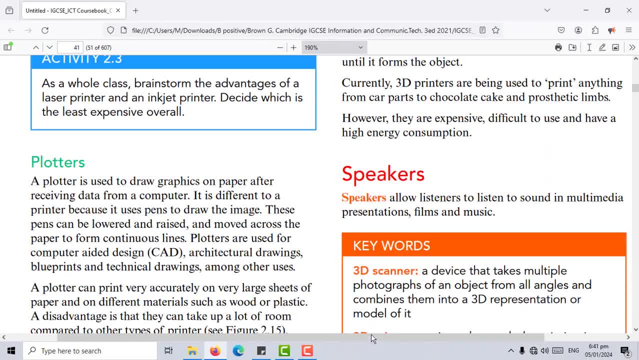 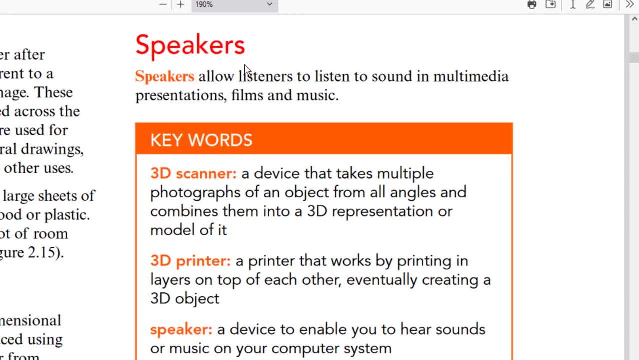 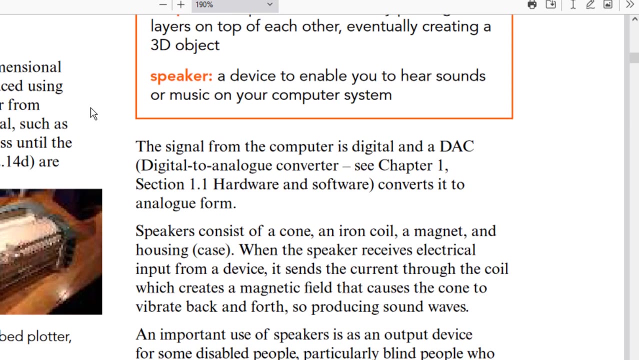 All right. so let's go to speakers, Which is like the easiest definition that one can just read one time and remember. speakers allow listeners to listen to sound in multimedia presentations, films and music, and that is it, All right. speakers allow listeners to listen to sound in multimedia presentations, films and music.